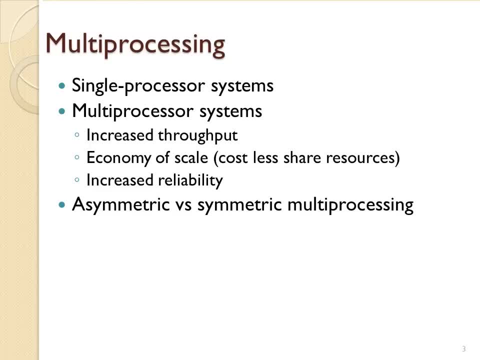 is the master and the other processors are slaves. So if you have an asymmetric setup, you will have assistance with your management with the processing units. If you have a symmetric setup, that means that all processors are treated as peers and all the management is done by the 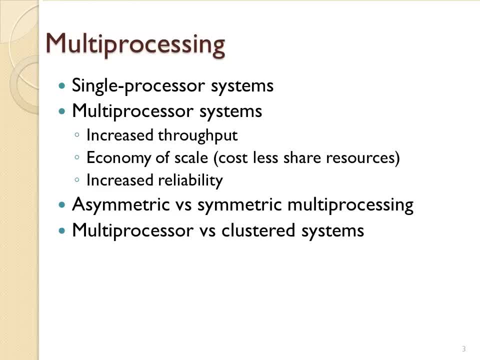 operating system. And one more thing about systems, multiprocessor systems. there are. in addition to having multiprocessor systems, there are clustered systems. Clustered systems are those systems that are separate computer systems. They have their own clock and their own resources, but they work together in some type of network as if they 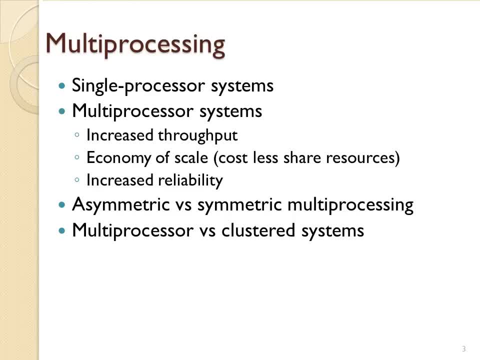 were one system. So again, there are different considerations on how the management is done in a single processor system, a multiprocessor system, a symmetric multiprocessor or an asymmetric multiprocessor, or a clustered system. And then the last topic I want to bring up is the 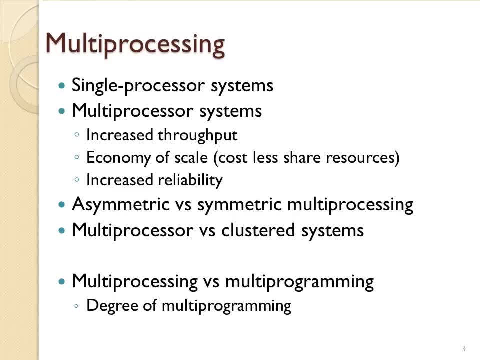 concept of multiprocessing versus multiprogramming. Multiprogramming is just a system that allows multiple processes to be active on the system at the same time. So you can do multiprogramming on a single processor system. you just need to switch between the processes and only do one thing at a time. You can also do multiprogramming. 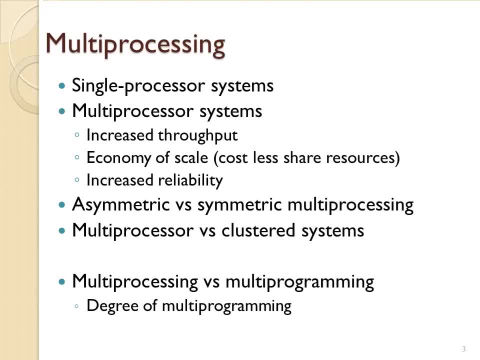 on a multiprocessing system, which just means you're using multiple processors to run multiple processes, And we will be discussing this term in a little bit, but I'm going to talk about it a little bit later in this course. this term, degree of multiprogramming, And there are 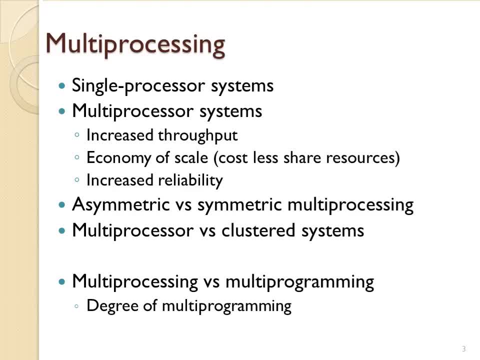 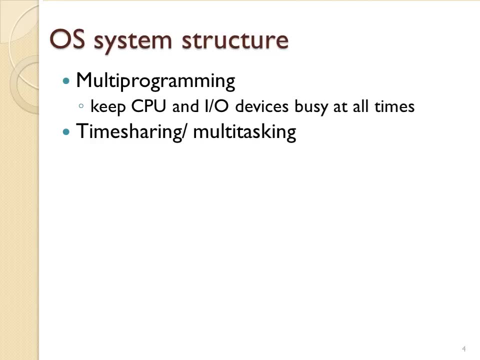 units that are part of the operating system that control the degree of multiprogramming And what that means. it controls how many active processes your system will allow at one time. So let's just talk a little bit about some of the goals for multiprogramming. In multiprogramming you have 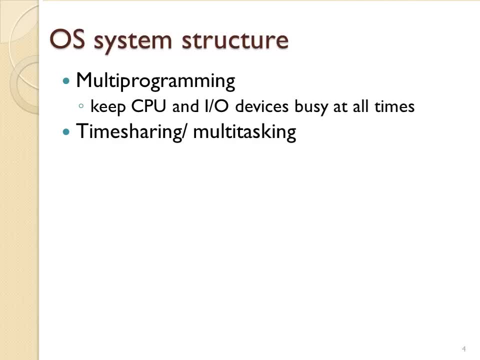 a bunch of processes and processes are. you know? you have a bunch of processes that are going to use the devices and use the CPU and use all of the resources. So what you want to have is a good mix of processes that are more CPU intensive and less CPU intensive, so that you 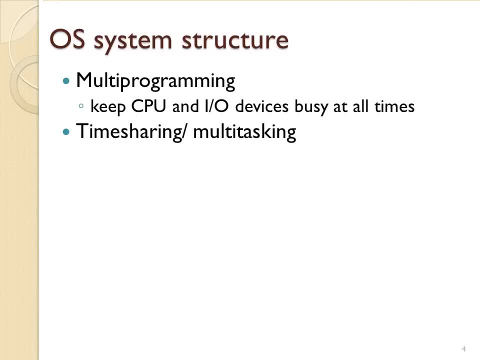 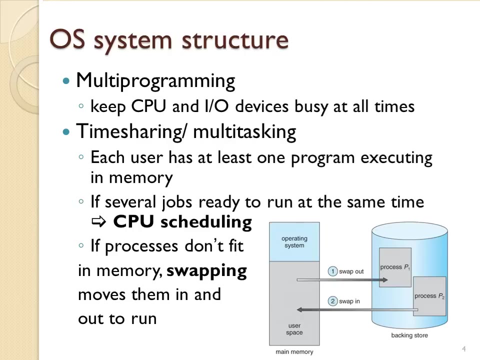 can keep all of your- all of your devices and your processor busy and get the tasks done with a good in a good amount of time. And then we have timesharing and multitasking systems And in this case they you need to have your operating system help manage all of these tasks on the system And 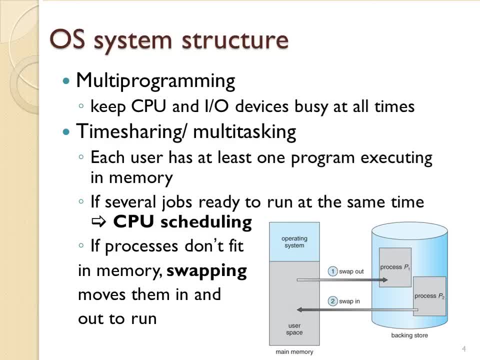 because we will have multiple active active programs. you will have a CPU scheduler and the CPU scheduler, which we will be doing a lot of exercises on that later in the course. But the CPU scheduler will take all of those active programs which are processes and are ready to get on the 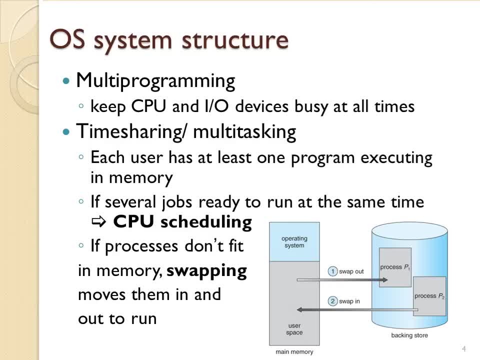 CPU And then we're going to have a CPU scheduler that will take all of those active programs and decide the order in which they get onto the CPU. And another part of the component of the operating system that that can control the degree of multi programming is if sometimes you know, you only 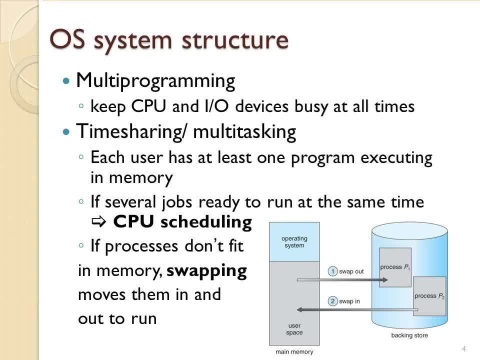 have a limited amount of resources. So once you have exhausted all of your memory in your system and you can no longer introduce any more tasks into the system, your operating system may have a unit that will swap, and it will swap either the operating system or the CPU scheduler, And so 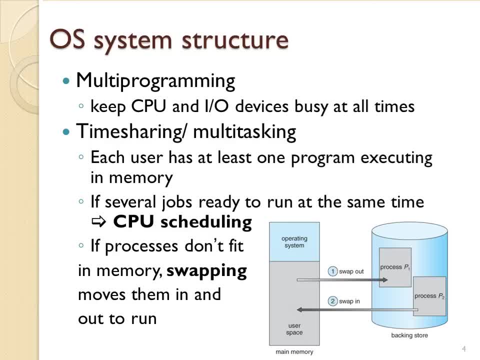 we're going to have a CPU scheduler that will swap either entire processes out of memory or parts of processes out of memory in order to give space for new processes to be introduced into the system, And we will talk about that when we get to schedulers and scheduling, So the components of an 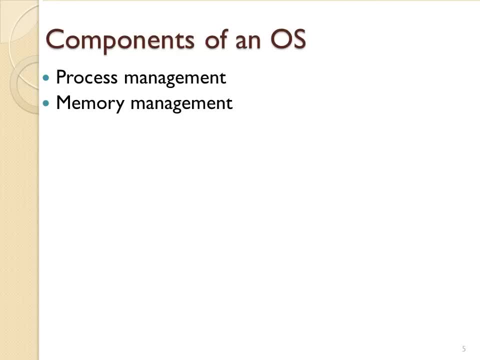 operating system. an operating system is a complex software, So in order to analyze it, we just talk about the different managers that are part of the system. we have a process manager, a memory manager, a storage manager that creates a uniform look to the system and manages all of the files and 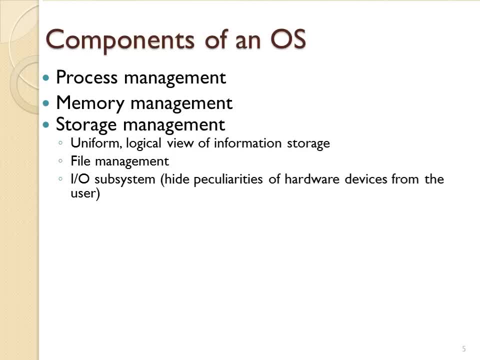 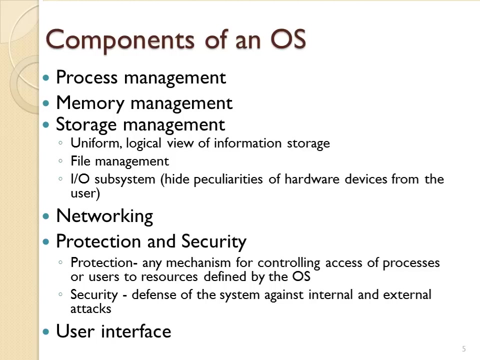 information and the kernel IO subsystem which manages the devices, networking, protection and security, And there's a definition here between protection and security: Protection is controlling access of the processes by the operating system and security is defense against attacks. And all systems will have part of the operating system. 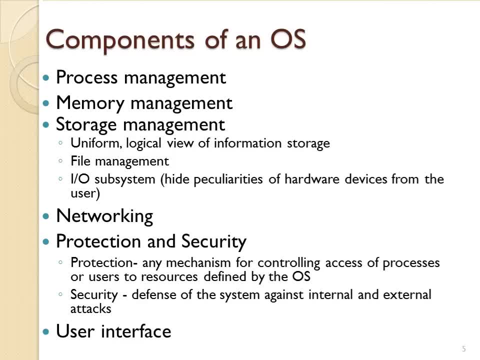 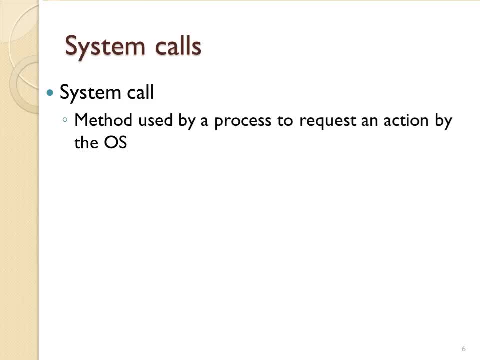 a way to interact with the system through a user interface. System calls are used by processes to request an action by the operating system. So what that means is there are privileged actions that are done on your system, like accessing files, allocating memory, communication between processes, and all of these tasks are done through system calls. 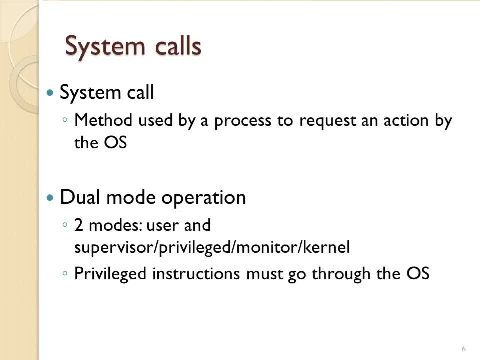 where the operating system will take over the system and not allow user processes to do anything. that is privileged. And one of the ways in which this is implemented is through dual mode operation, where you have two modes of operation In your system. you have user mode, which the application. 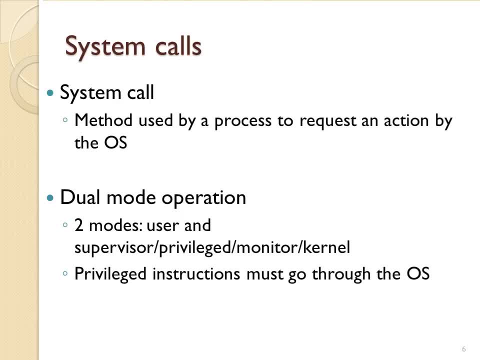 is run in. and then you have privileged Kernel mode or supervisor mode or monitor or kernel. these are all or privileged. these are all interchangeable. You only have two modes: user mode and the privileged mode, which is the kernel mode. 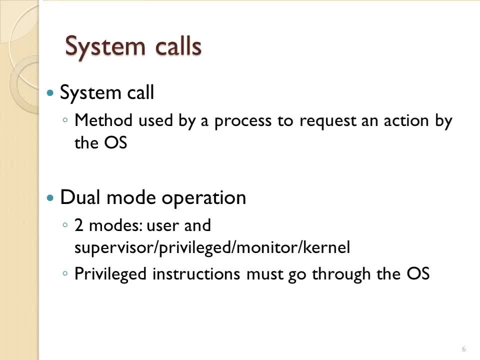 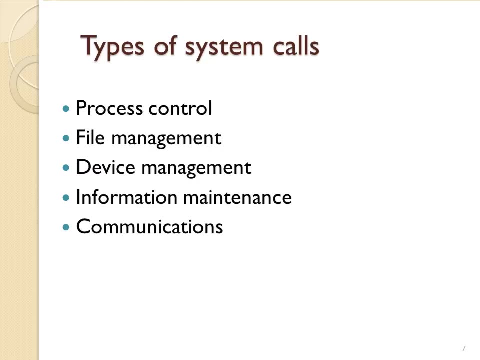 And all privileged instructions must go through the operating system and give control to the operating system to do any of these types of operations. And the different types of system calls include those that for managing processes, for managing files, for managing devices, for updating information and for managing communications. 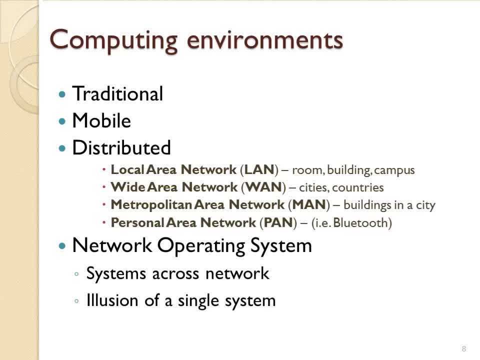 And the last topic I want to go over in this section is different types of computing environments. So when you're dealing with operating systems and this manager of your computer system, it not only depends on whether you have what the components of the software are and how you have set up your system calls and all of that. 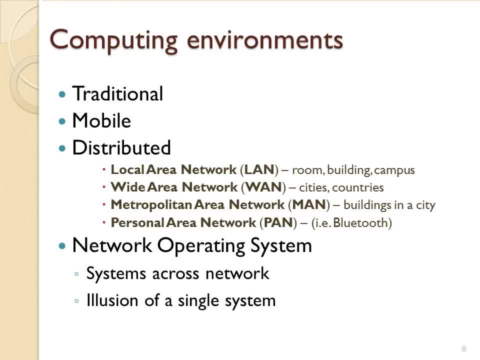 but it also depends on what type of system you're actually using. If you're using a traditional computer system where you're just using your own computer and you are doing word processing and doing independent work on your system- and that's very different than a computer system that is getting connected to the network and is having to deal with, you know, security issues, because you're on a network and you are downloading stuff and all of that.